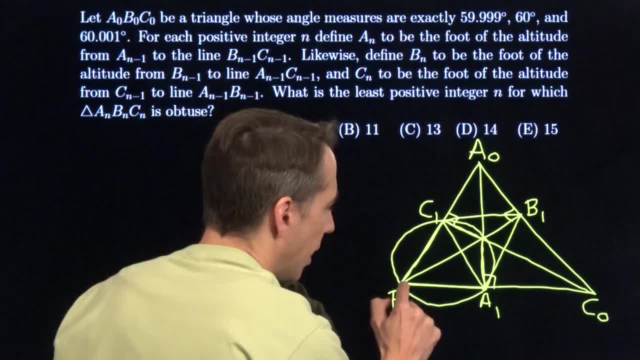 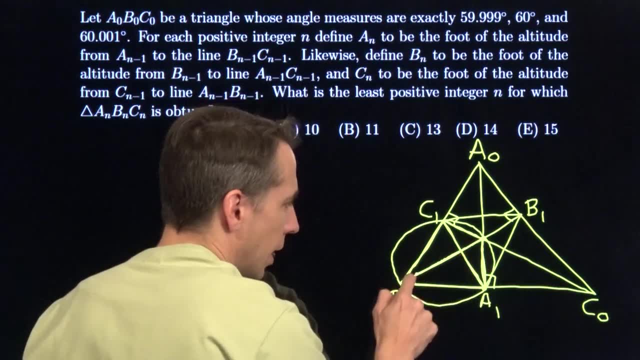 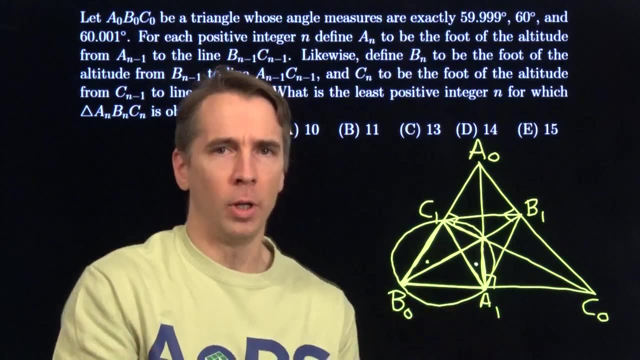 C-1, so I'm going to focus on this and this, And I see this angle is inscribed in the same arc as this angle. So these two angles are inscribed in the same arc. that means they're equal. But this angle out here is part of a right triangle. This right triangle right. 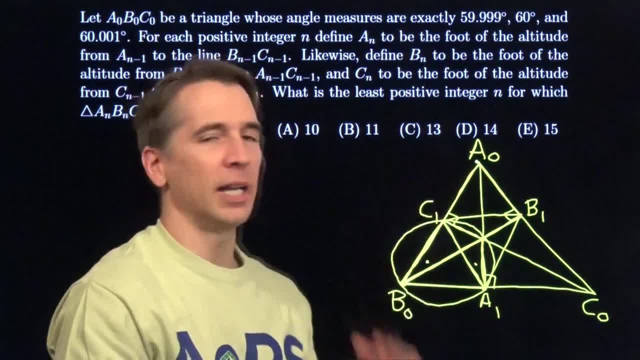 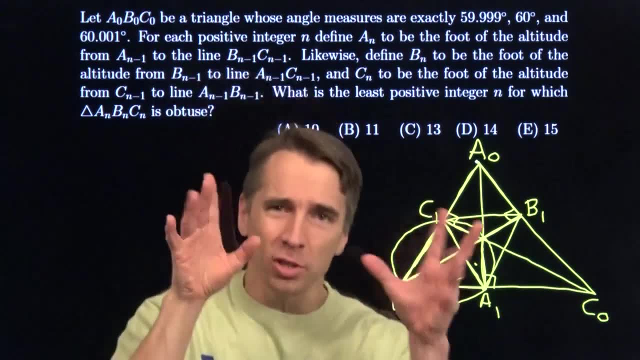 here. So this angle is 90 minus A-naught, which means this angle is 90 minus A-naught. Now, when I find something new in a geometry problem using some technique, I try to use that technique again because maybe it has more to give. So I'm going to take this whole. 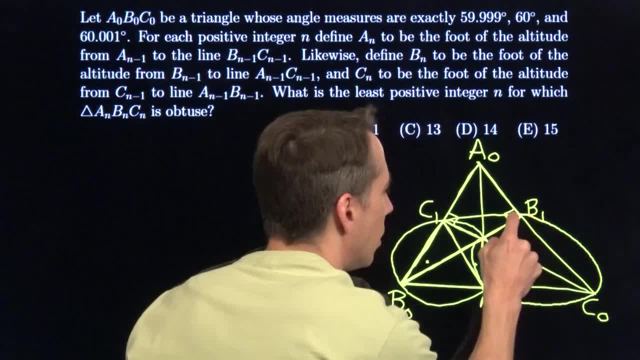 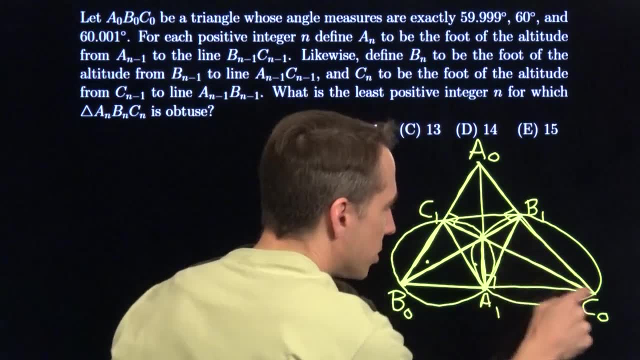 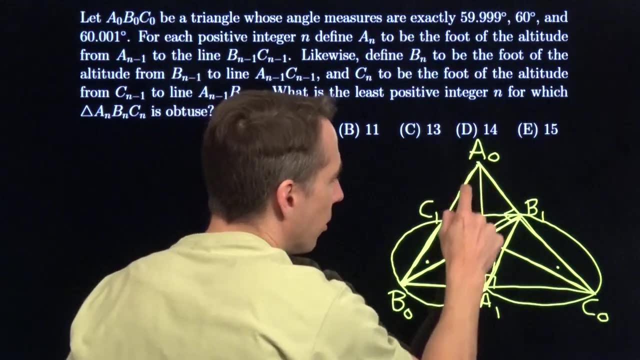 angle here, C-1,. I'm going to move it over here. draw me another circle. Now I'm going to focus on this angle and this angle. These two angles are inscribed in the same arc, so they're equal. This angle equals this angle And this angle is part of this right triangle. 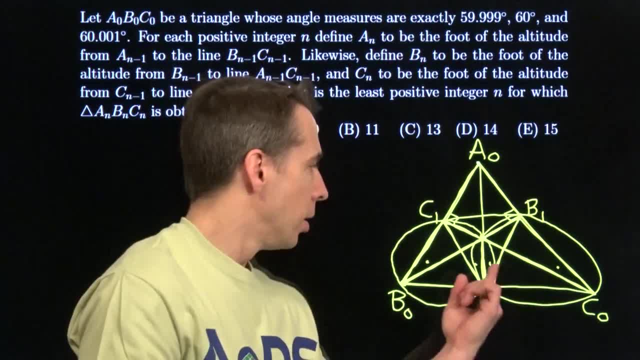 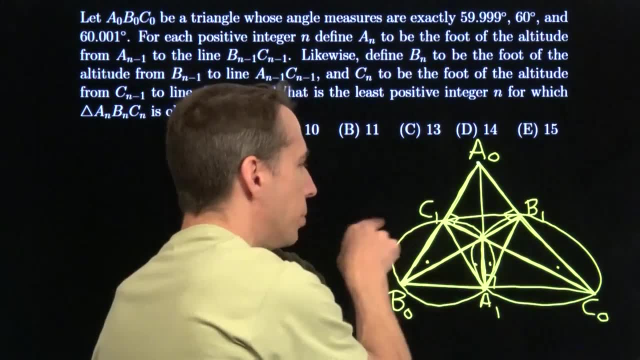 So this angle is also 90 minus A-naught, which means this angle is 90 minus A-naught. So you've taken the angle at A-1.. In triangle A1, B1, C1, split it into two pieces. both pieces equal 90 minus A naught. 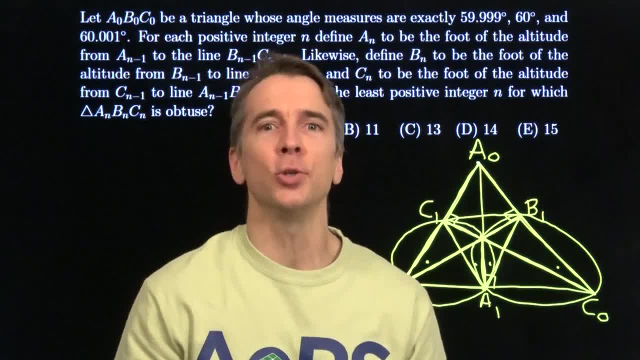 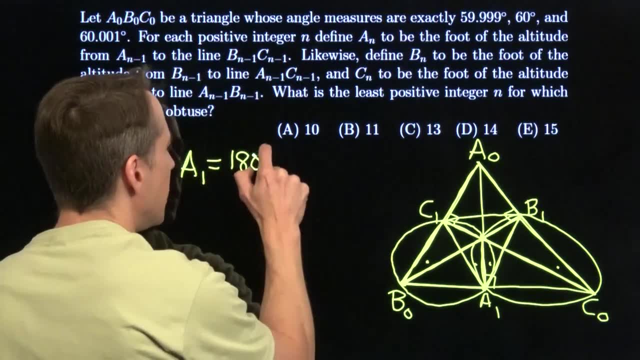 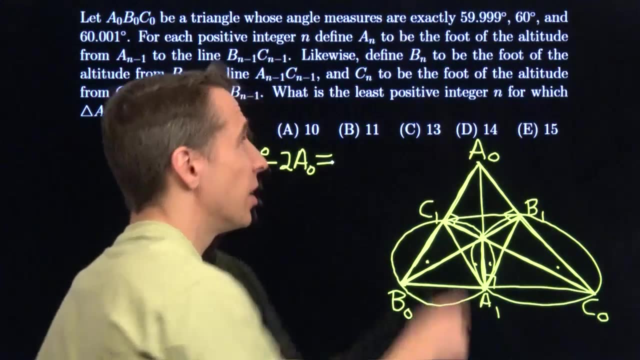 Put those pieces together, you get 180 minus 2 A naught. So now we can find A1. A1 is 180 degrees minus 2 times A naught. Now I'm going to take these three measures they gave us. I'm going to call that A naught. 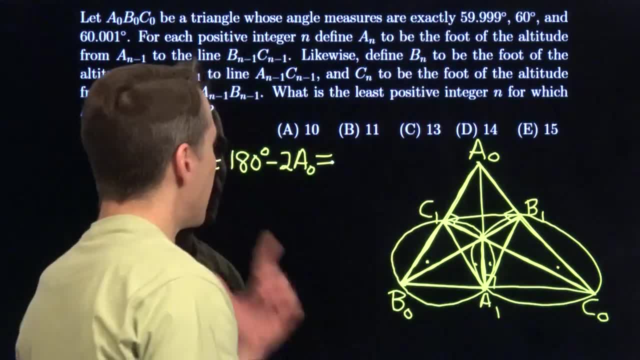 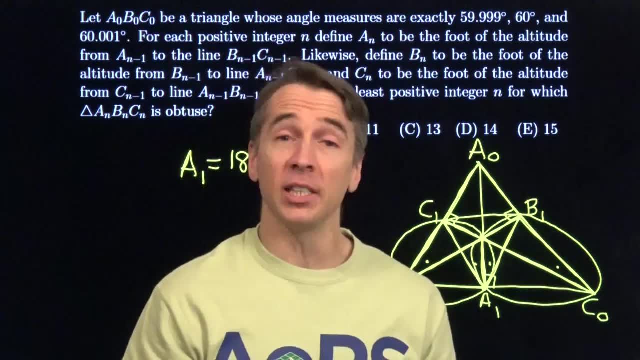 that B naught, that C naught. So we're going to double this and subtract from 180.. Now this is one-thousandth less than 60. So you double that, you get something that's two-thousandths less than 120, and you're. 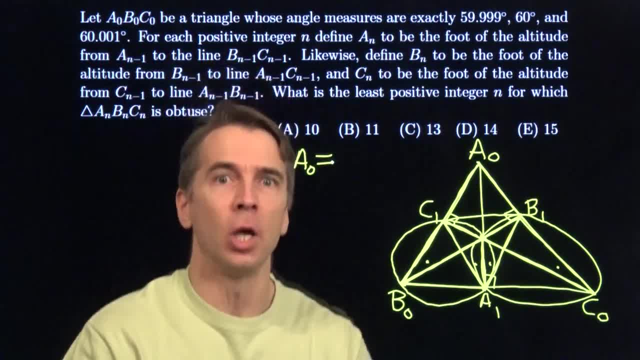 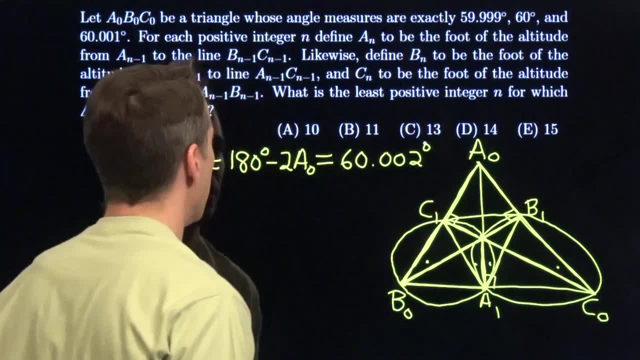 going to subtract that from 180, you get something that's two-thousandths greater than 60. You get 60.002 degrees. Now do the same thing with B1, I'll draw a bunch more circles, but we know what we're. 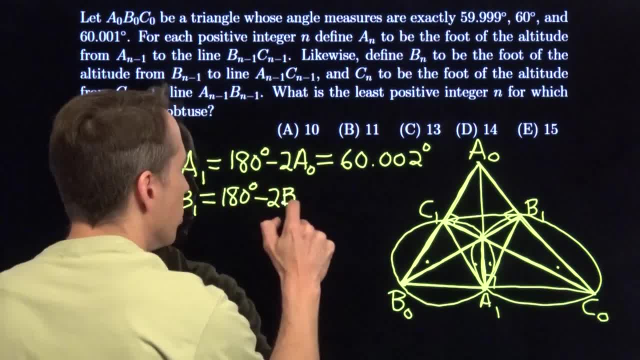 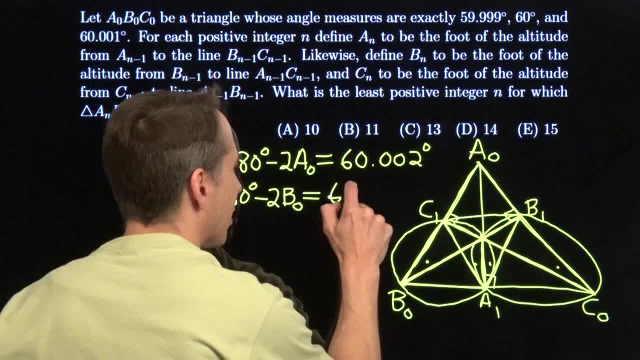 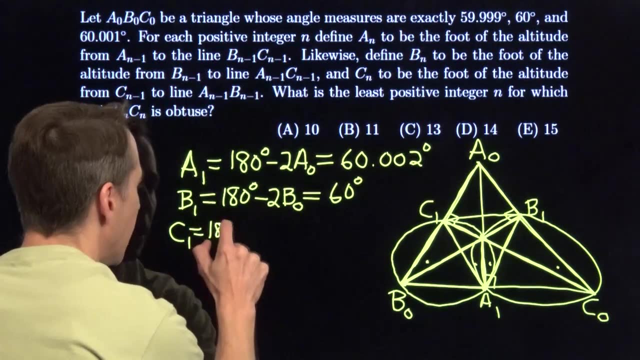 going to get. We're going to get 180.. 180 minus 2 times B naught, but B naught that's 60, 180 minus 2 times 60, you get 60 back. Now we're going to do the same thing with C. You know what we're going to get there. 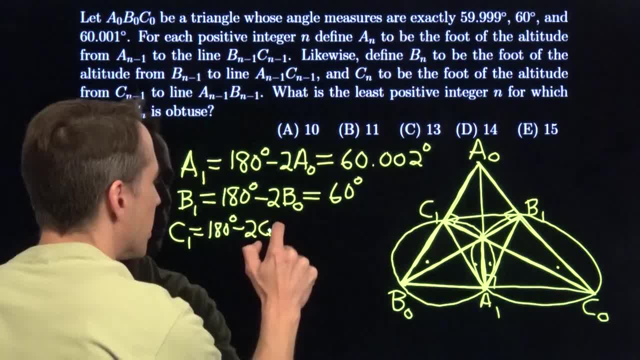 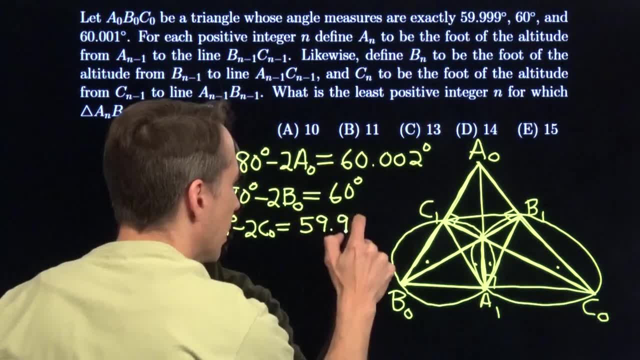 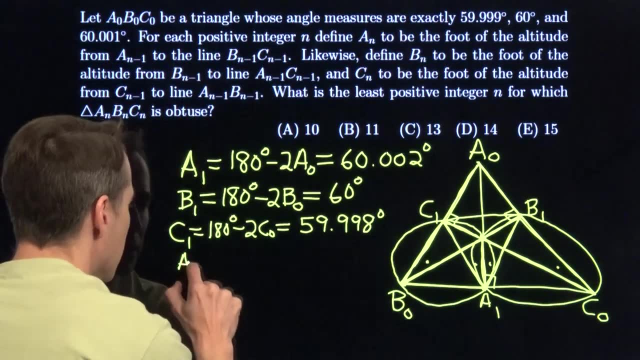 180 minus 2 times C naught. and we can go through the arithmetic or we can just look at these two and we can see that that last angle is 59.998.. Just use this same process to get to A2, B2, C2.. 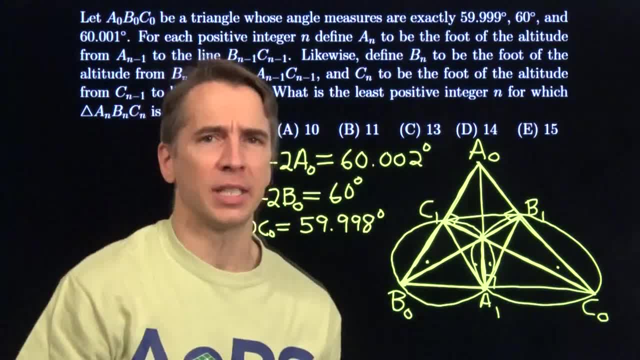 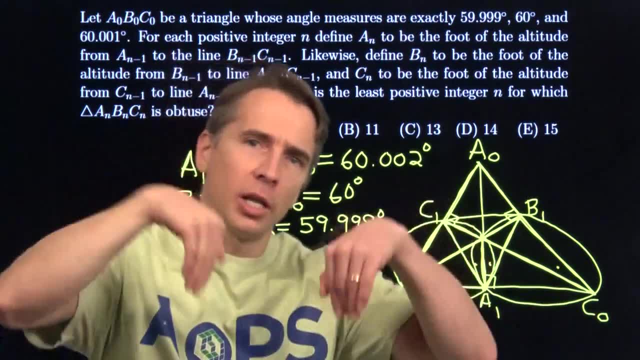 For A2, we're going to take that two-thousandths greater than 60, you double that, you get four-thousandths greater than 120, subtract that from 180, you're four-thousandths less than 60.. 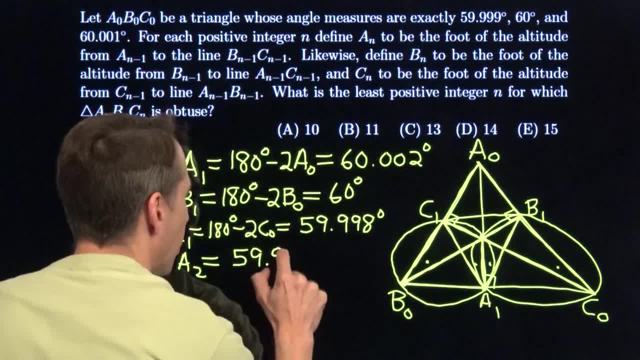 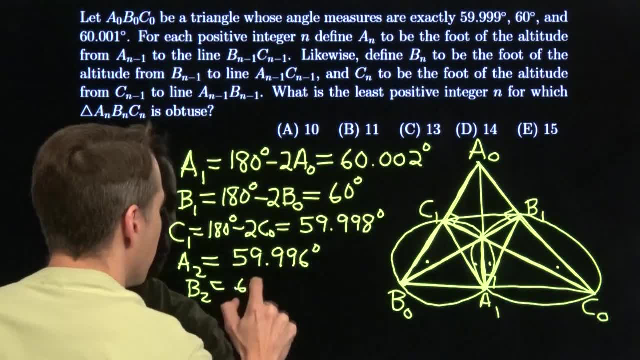 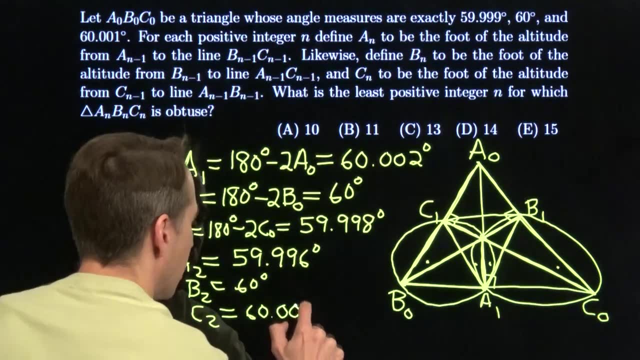 You're at 59.996.. B Still at 60. And C 50.996.. C now is going to be four-thousandths above 60. And now we just have to keep doing this over and over and over again until the largest. 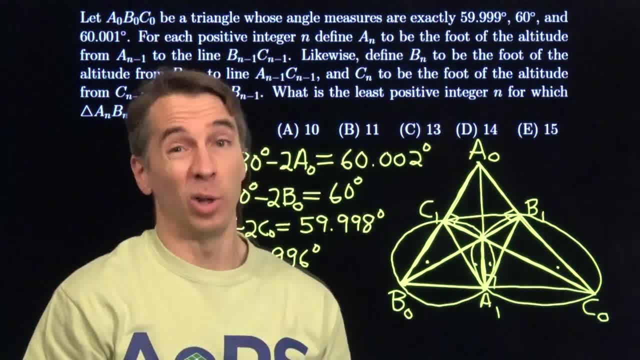 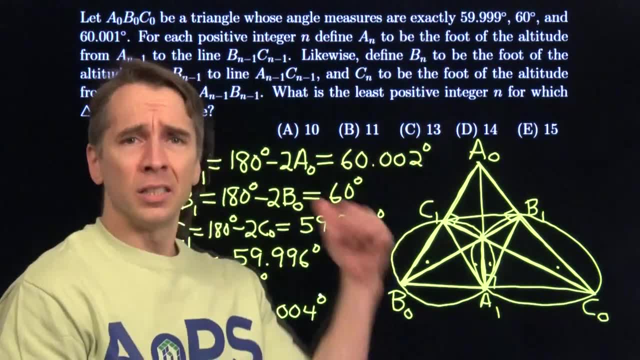 angle in our triangle is greater than 90. Now we could actually just do this over and, over and over again, but we're not going to, because we saw, as we were going from A naught to A1, and then from A1 to A2, what's actually. 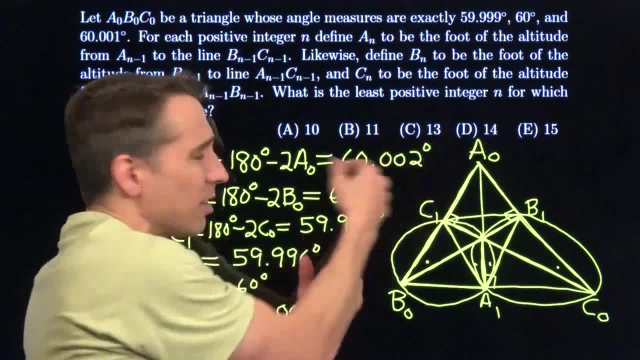 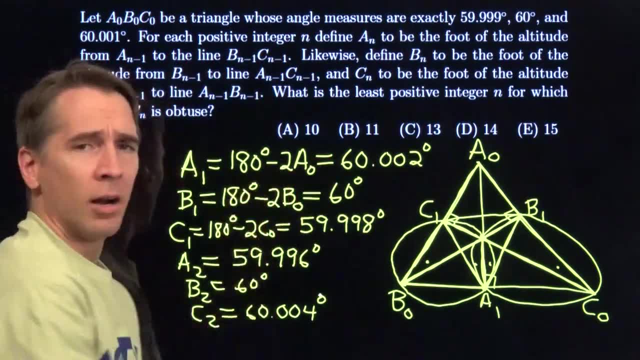 going on here. The difference between each of these angles, it's not 60 and 60. Those differences just doubles at each step And we saw why It's right there. It's right there. Our largest angle here was two-thousandths greater than 60.. 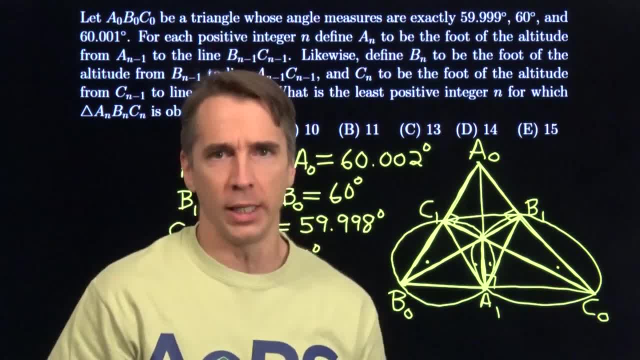 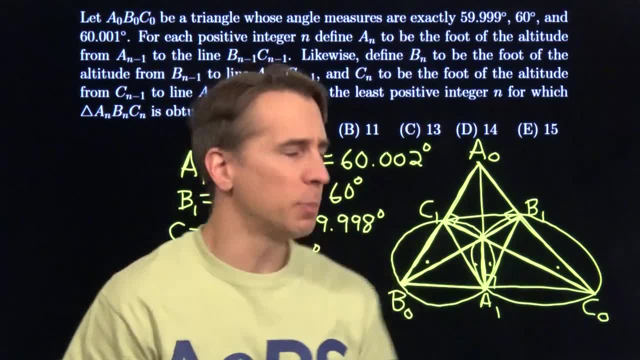 And then we doubled that You're four-thousandths greater than 120. Then you subtract from 180 and now you're that four-thousandths away from 60. So at each step, the difference between the two angles that aren't 60 and 60 itself, that 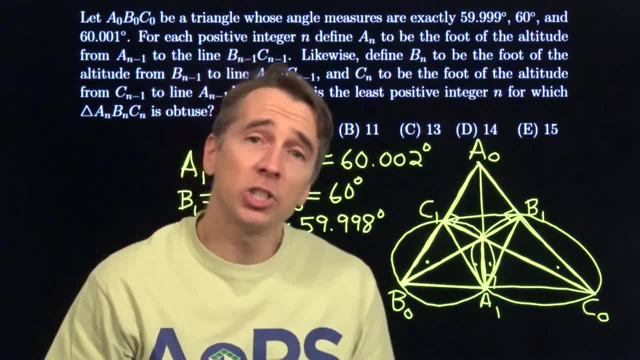 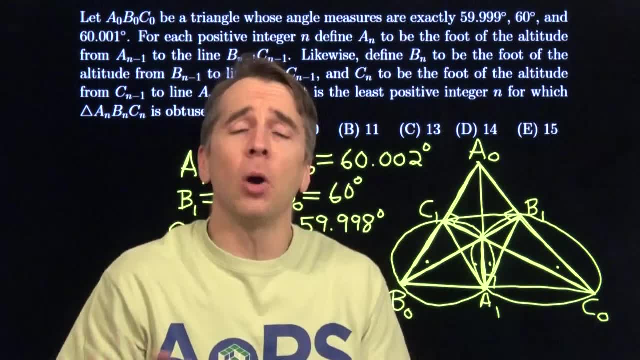 difference just doubles at every single step. And we started off one-thousandth, One-thousandth away from 60. Double that, You get two-thousandths, Then four-thousandths, Then eight. We have to keep going until our total difference between that largest angle and 60 is greater.